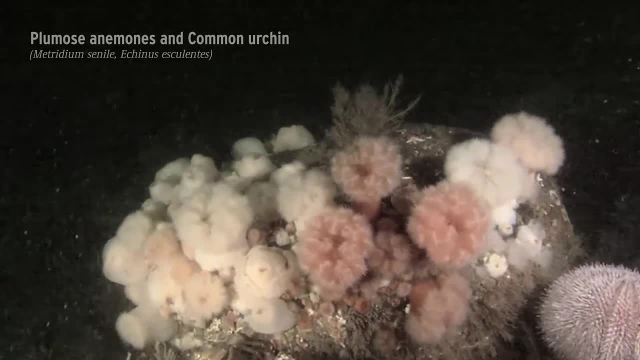 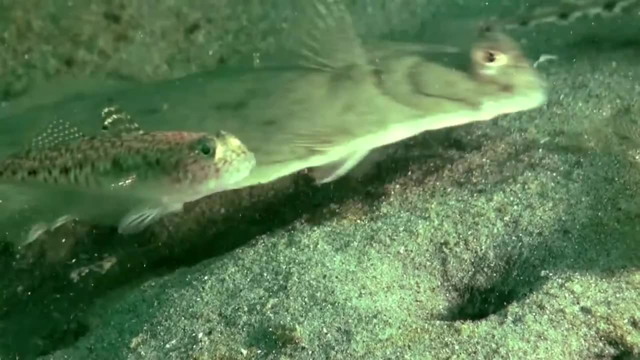 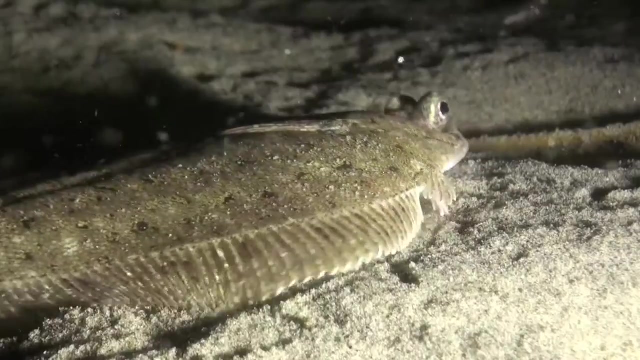 many endangered species live on the reefs there and on the sands of the amrum bank, a rearing ground for various kinds of fish. these provide sufficient food for harbor porpoises with their young and for seabirds. the biggest sandbank in the north sea is dogger bank, which is 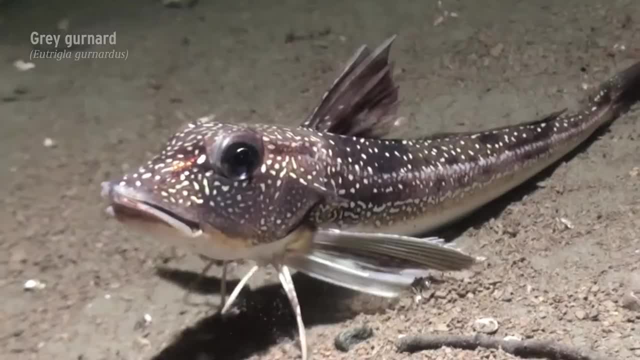 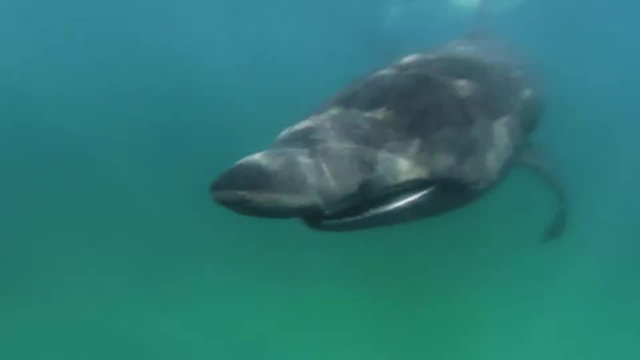 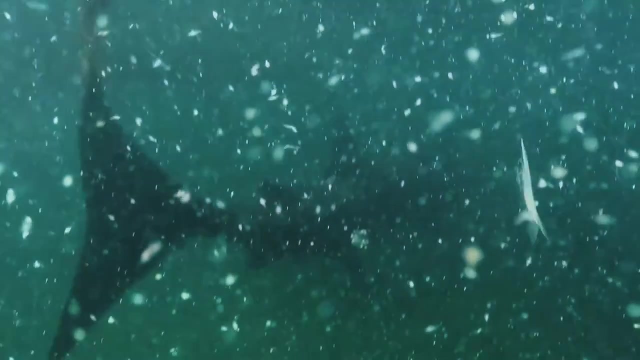 exceptionally rich in fish species- the natura 2000 mpa is set up here by three different countries- are visited by a whole selection of whale species and even the basking shark, a plankton eater. in the quest for food, these impressive sharks migrate along largely unknown routes through the north sea. 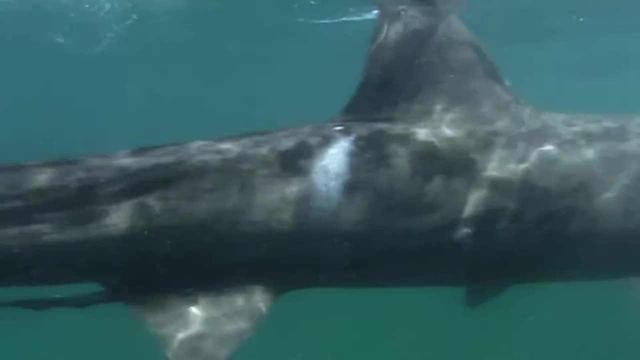 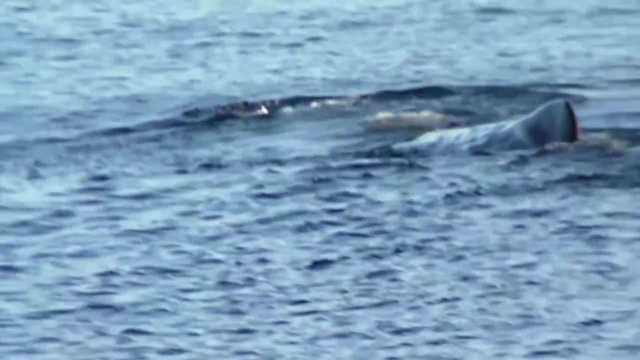 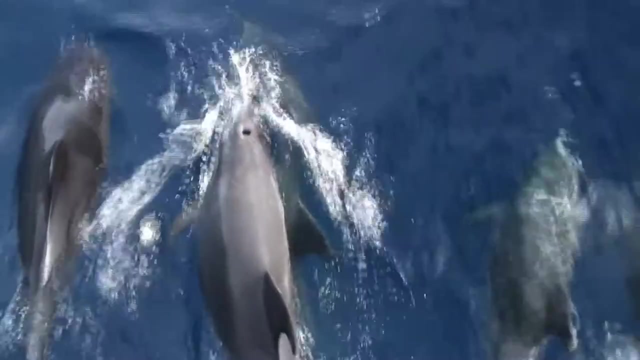 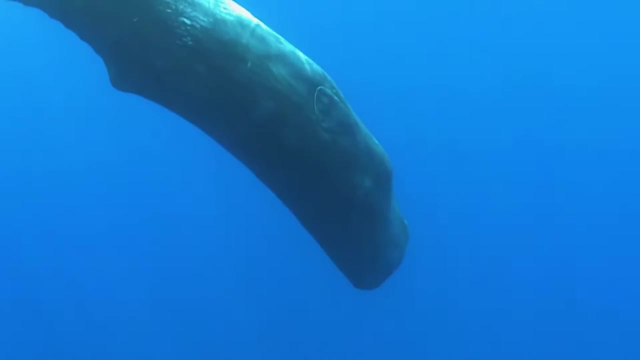 and evidently through the north sea, and evidently through the north sea, the channel to the southwest coast of england. other migrating species too, like sperm whale and dolphins, need wide-ranging protection along their migratory corridors and in favored breeding and feeding areas such as around the azores. 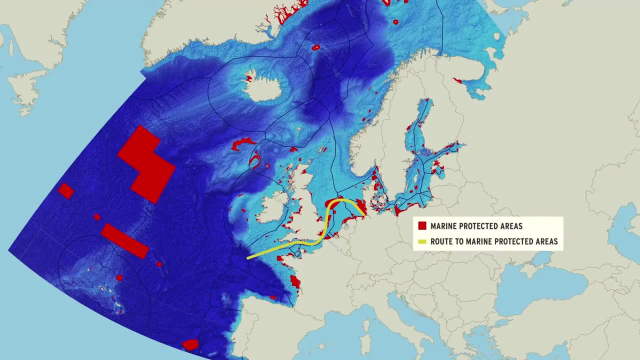 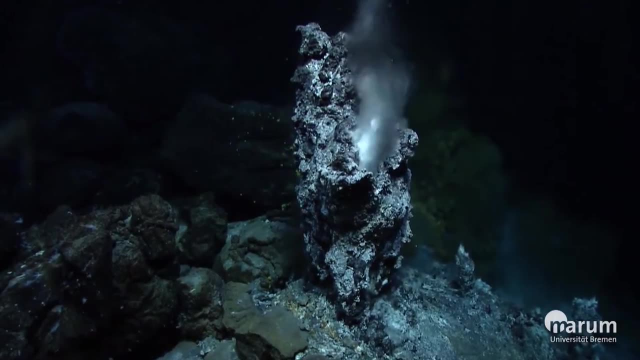 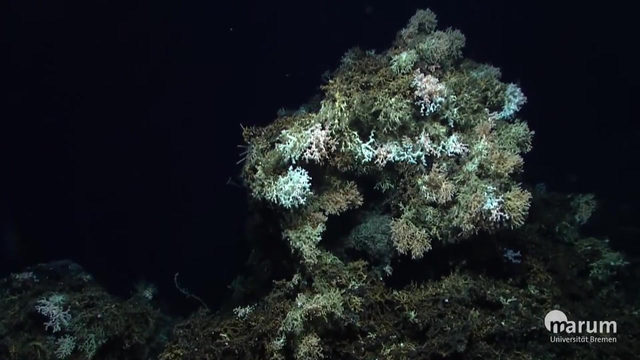 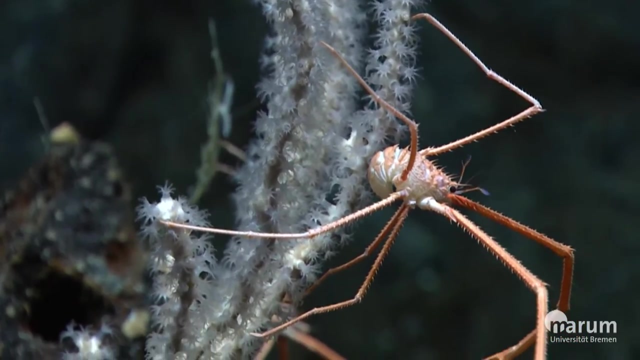 the azores are an archipelago on the mid-atlantic ridge, a highly active volcanic zone. hydrothermal vents and gas seeps are found here, many hundred meters down. they are home to very special ecological communities with countless rare deep sea species. stony corals like laphelia and madrapora, together with gorgonians, form unique cold water coral reefs. 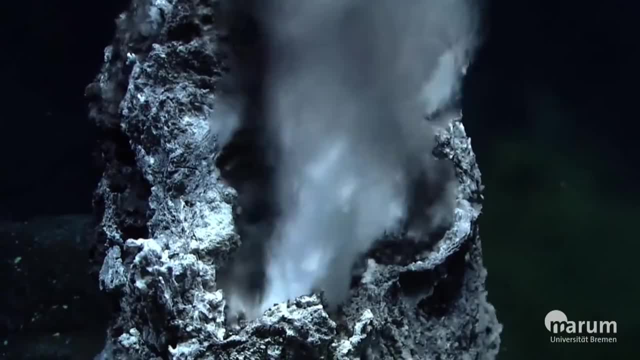 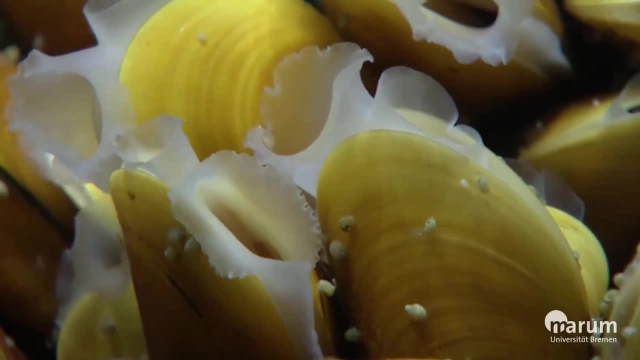 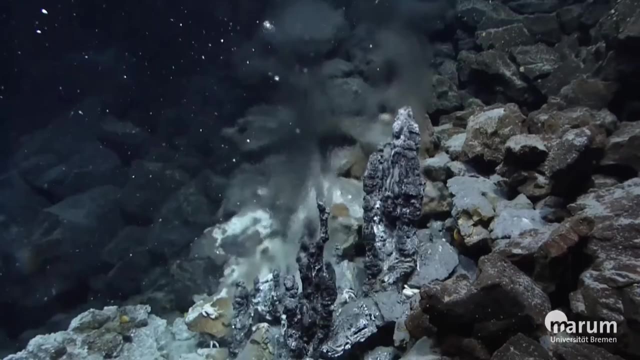 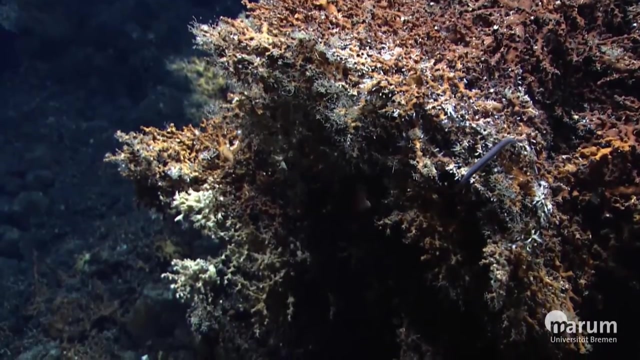 deep sea mussels directly colonize the hydrothermal vents. they are specialists in this extreme environment, as are deep water crabs. portugal has put several of these valuable areas under protected status, but many unusual deep sea habitats are outside any national jurisdiction. intensive global efforts are underway to identify and assess these areas of outstanding. 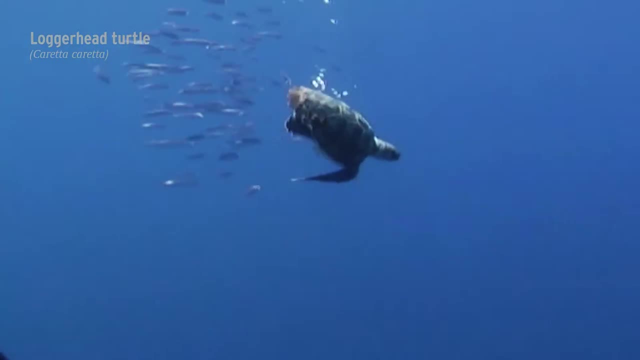 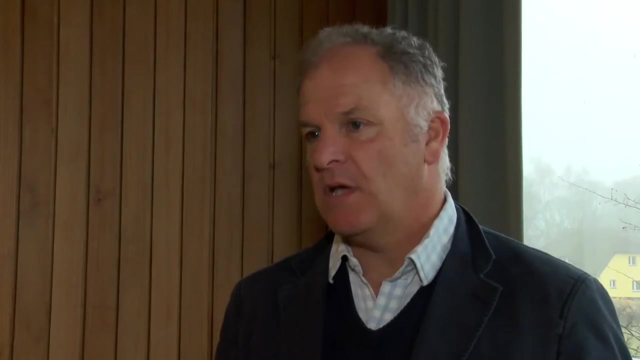 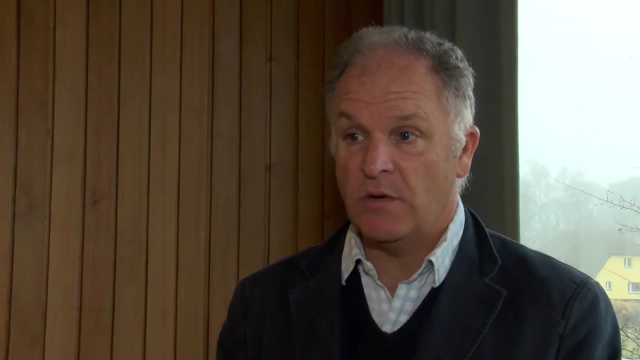 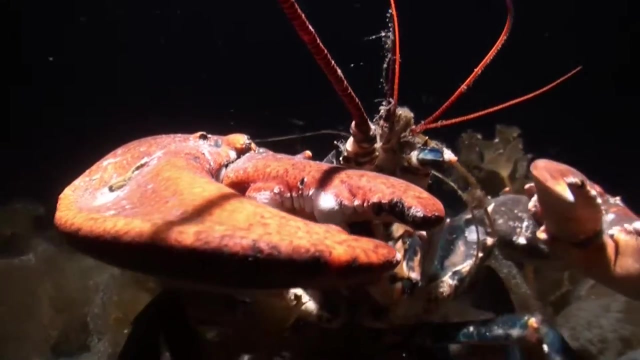 ecological value. part of this work is gobi, a project with bfn funding. gobi is a collection of partners, of organizations around the world who are working on collecting information on biodiversity, so it's providing physical and biological data to to organizations like the convention on biological diversity that are keen to protect biodiversity. 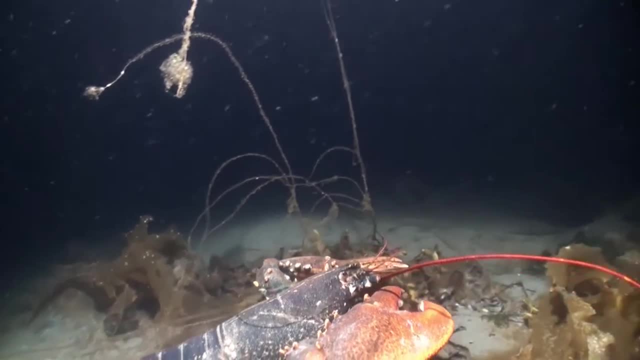 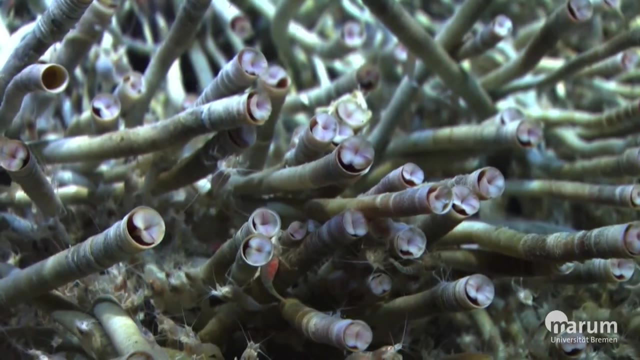 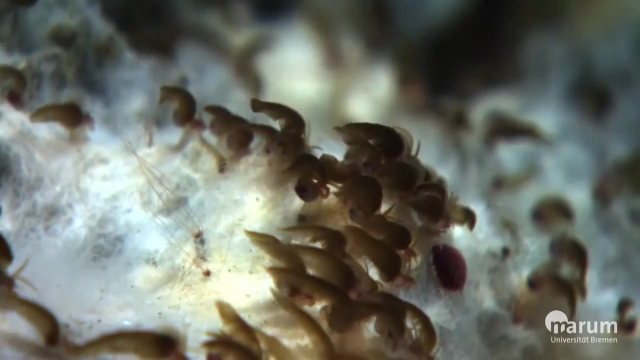 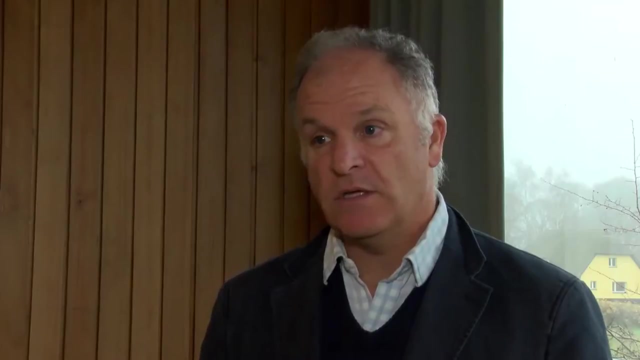 and initiate marine protected areas, but also these ecologically or biologically significant areas. so gobi partners have been instrumental in the regional workshops to provide data, to provide advice and expertise to state parties and to organizations that might bring together some of the most important research projects in the world. 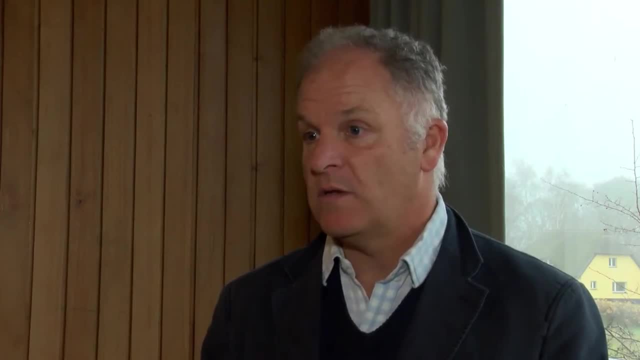 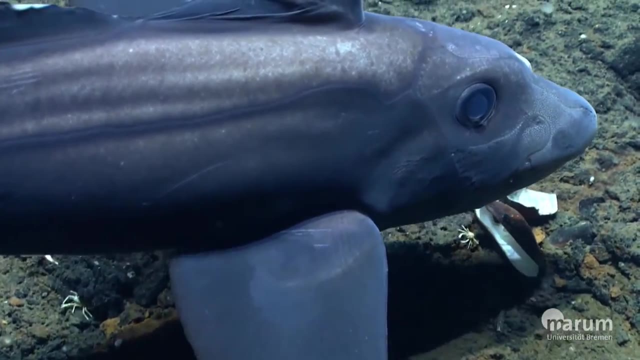 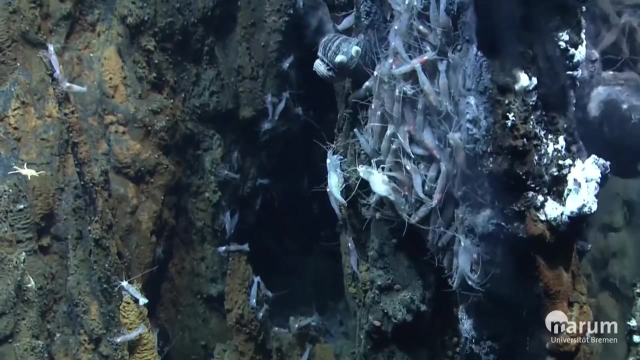 i think that's been a fundamentally important role that uh, bfn and germany have played into providing some funding that helps collate this information. assessing and designating epsos- ecologically or biologically significant areas- across the various marine regions- is a complex process involving regional workshops all over the 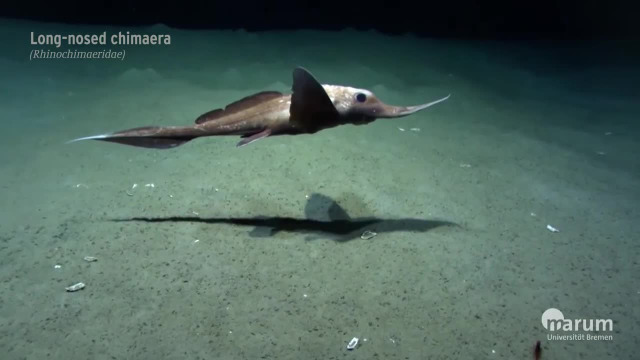 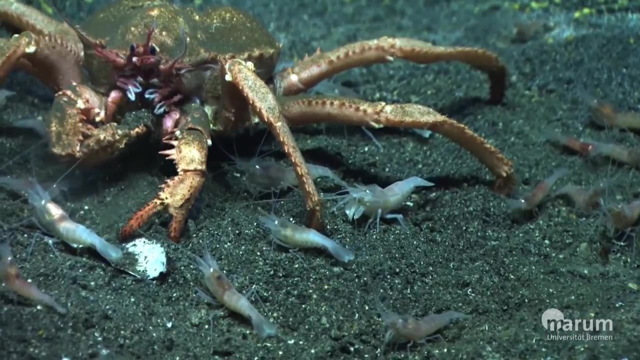 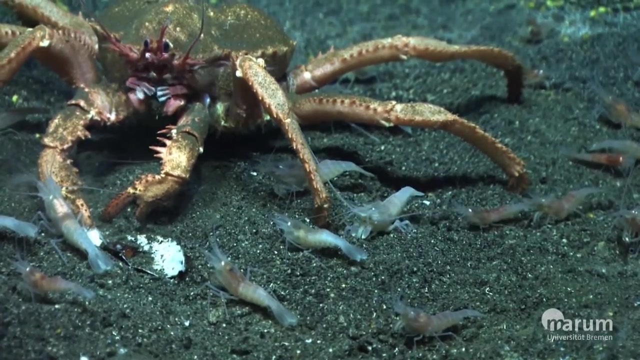 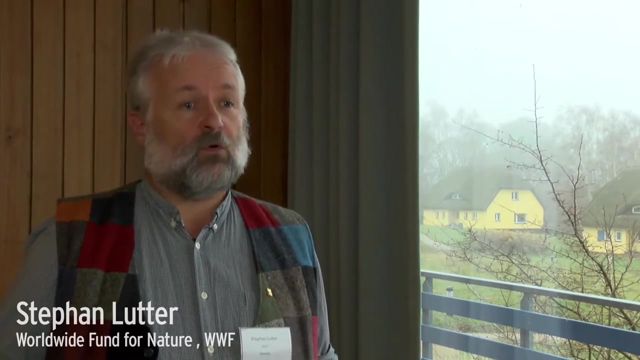 world. some 200 epsos have been identified so far. their final designation is decided on by the parties to the convention on biological diversity. identifying epsos- so-called ecologically or biologically significant areas in the world oceans- is important, especially in regions outside ospar, where we do not have a lot of 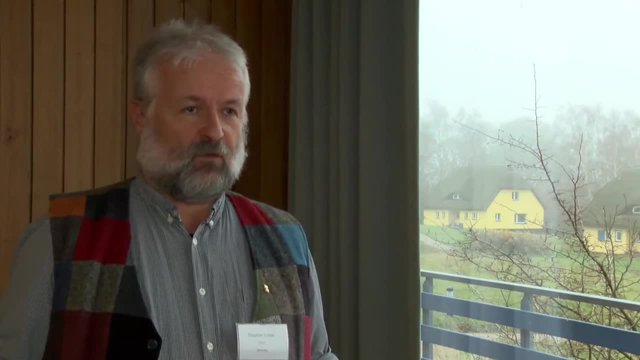 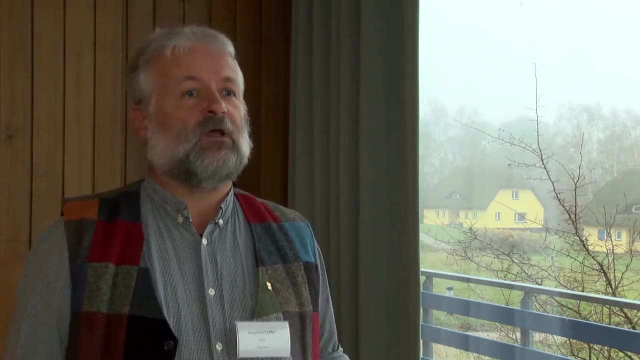 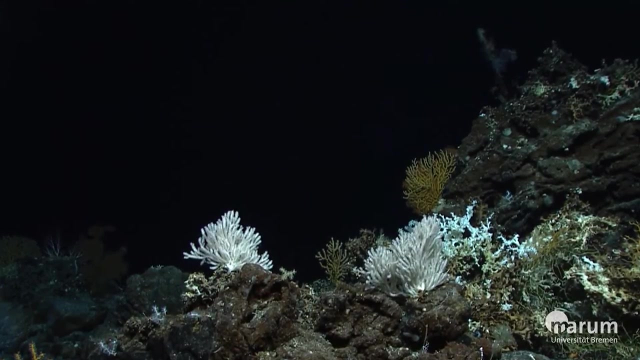 we do not have a governmental intergovernmental framework for mpas on the high seas and in remote areas at sea, so they serve as kind of precursors for mpas, potential mpas for the future, and we as an ng o propose epsos also in the 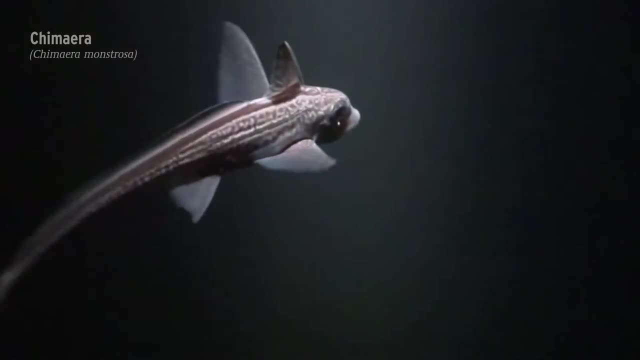 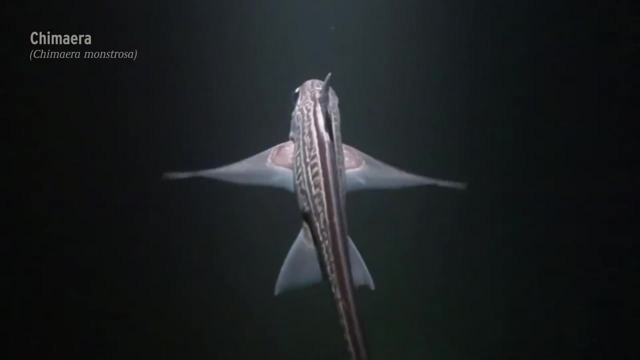 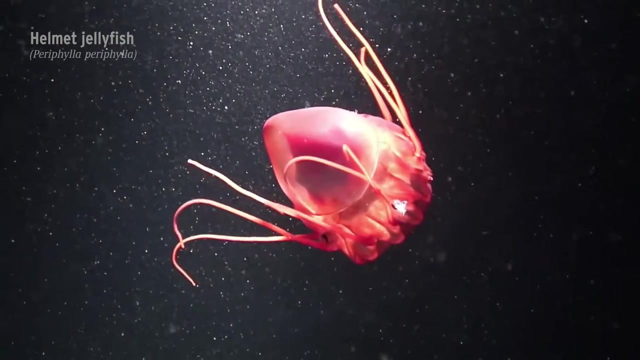 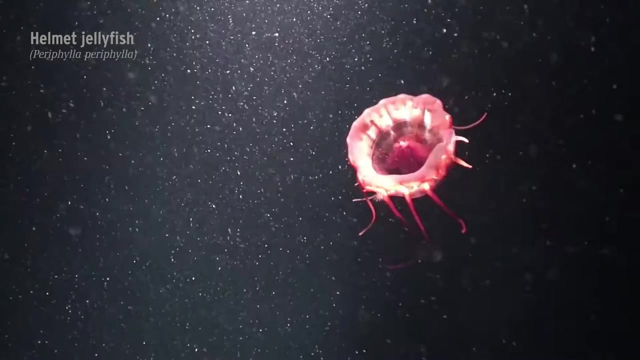 ospa maritime area where we see there is a gap, but others adjust. the first step, turning them into globally respected protected areas. most regions outside of national jurisdiction takes good international cooperation. Germany's Federal Agency for Nature Conservation is involved in many of the bodies set up to designate MPAs. A leading example is the Charlie Gibbs MPA. 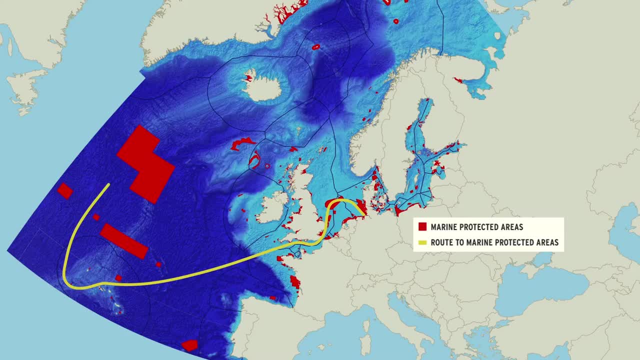 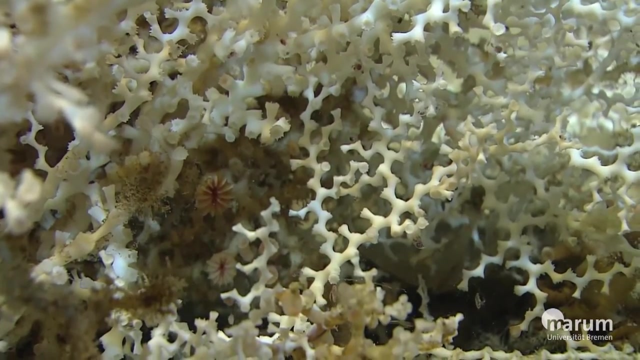 in a fracture zone on the Mid-Atlantic Ridge. With support from BFN and originally initiated by the WWF, scientists have identified exceptionally valuable areas within this zone: More than 40 species of cold-water coral, including Lophelia Madripoora. 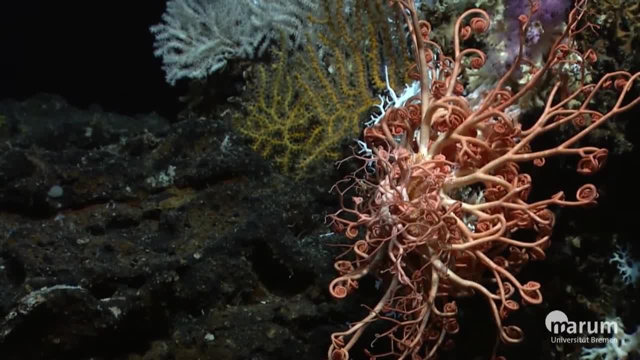 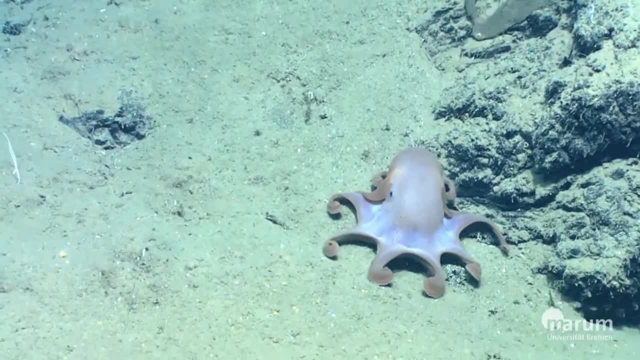 and Gorgon's Head are found here at depths between 700 and 4,500 meters, Likewise some 80 species of cephalopods, like the deepwater Dumbo octopuses. The osprey is one of the most important species in the world. 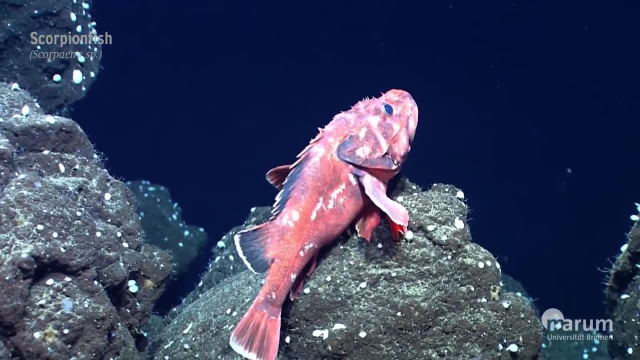 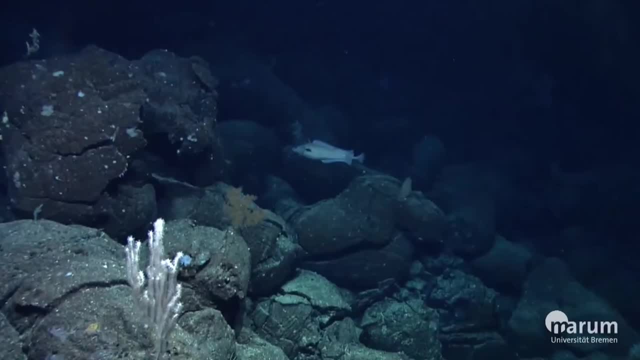 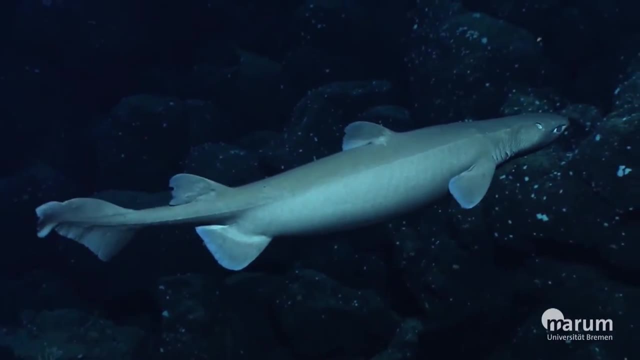 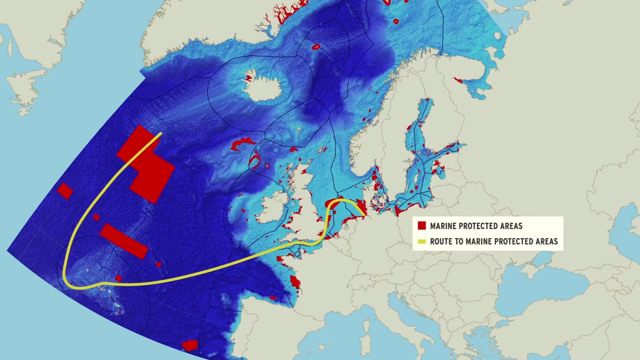 The OSPAR states agree to designate an area of 324,000 square kilometers. The MPA is home to fascinating ecological communities. There are dozens of fish species, including 40 species of deepwater shark alone, like this kitefin shark. The goal is to build a network of representative and well-managed MPAs across the whole of the 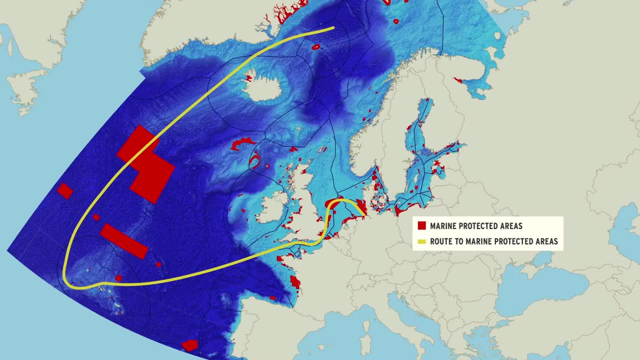 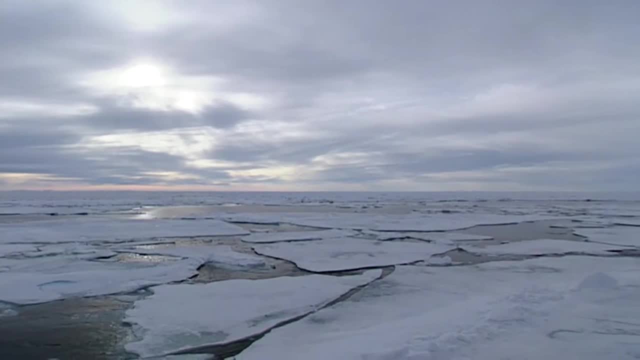 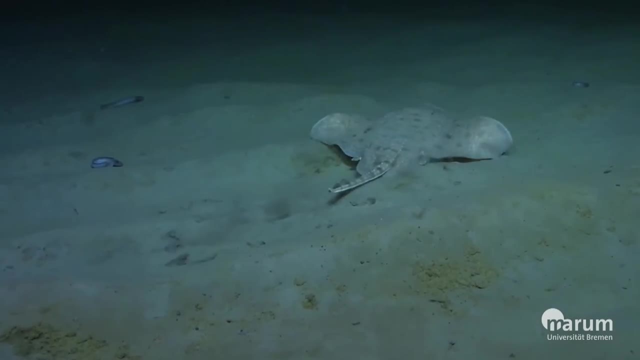 OSPAR area. About 5.2 percent of the Northeast Atlantic is protected so far, but there are still gaps. for example, in Arctic waters. While there are coastal protected areas, there is no widespread protection for areas far offshore. This makes effective management hard to implement and monitor. 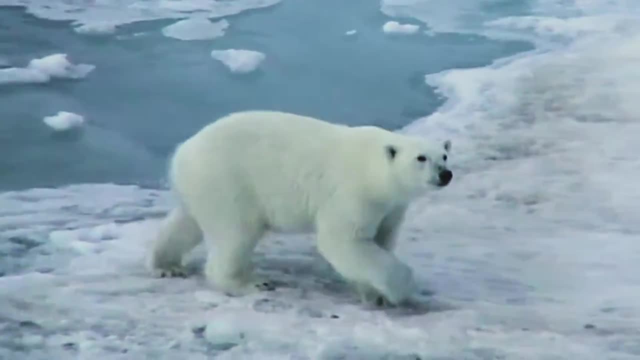 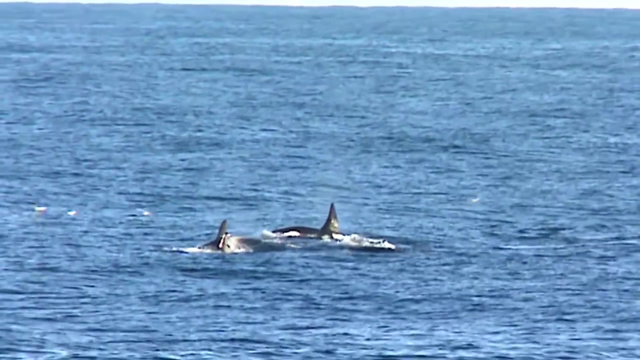 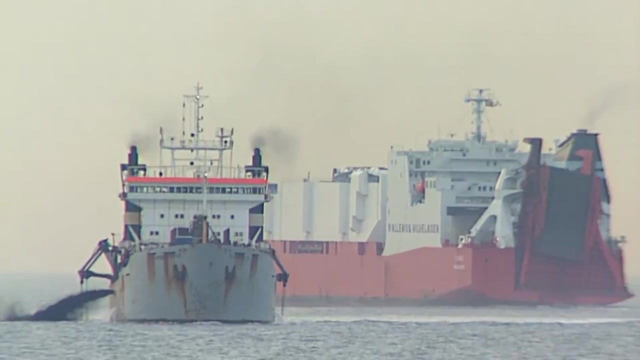 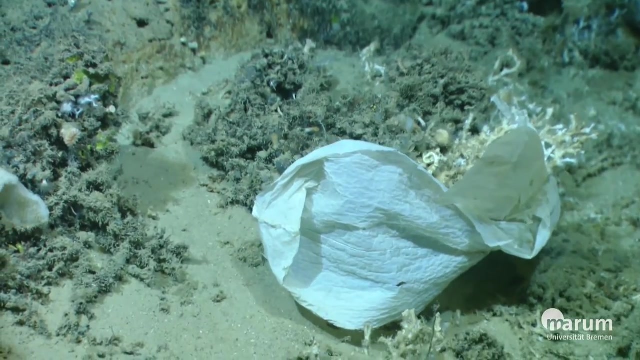 Yet these areas, too, are home to endangered species that have adapted to conditions in the icy waters, Together with ecologically outstanding and highly sensitive habitats. Even these remote areas are exposed to human pressures. Plastic waste and parts of old nets are a major threat to the marine food web. 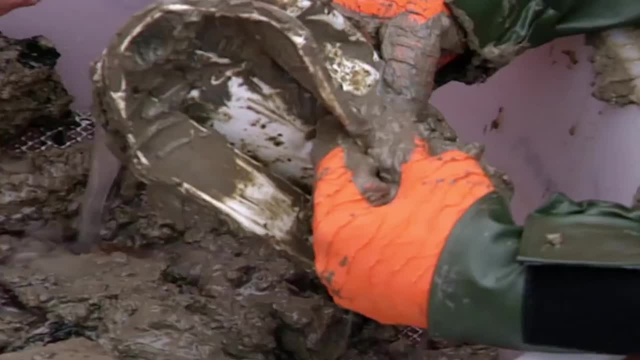 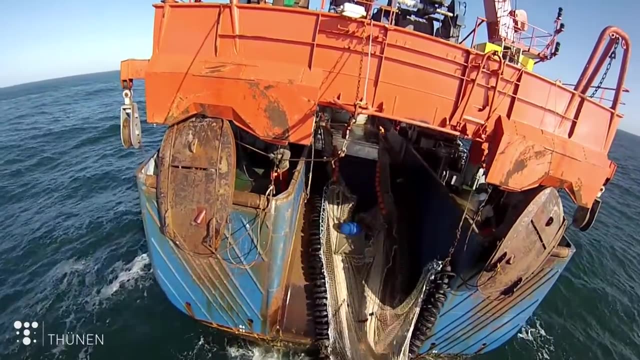 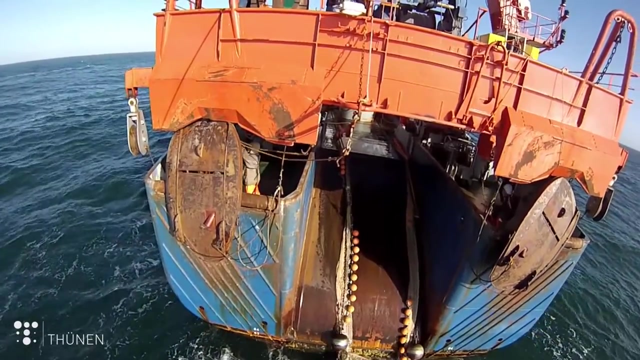 The debris of our civilization is found from the Mediterranean to the Arctic Ocean. At least 1,000 species of this species live on the coast, But it's modern fishing practices that do some of the greatest harm. The expansion of fishing grounds across the high seas poses huge risks. 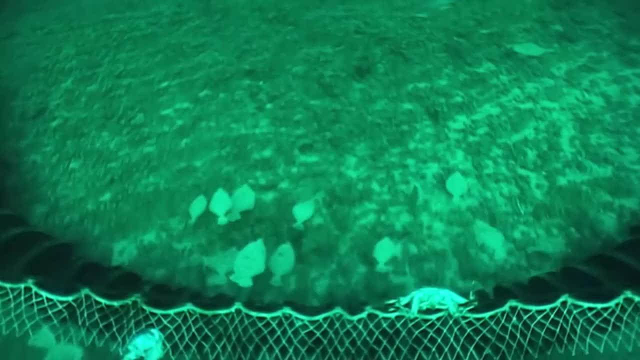 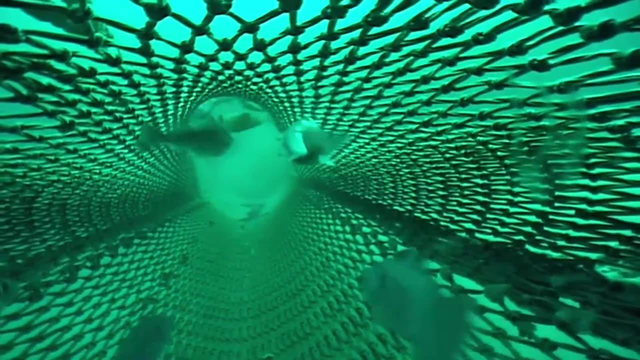 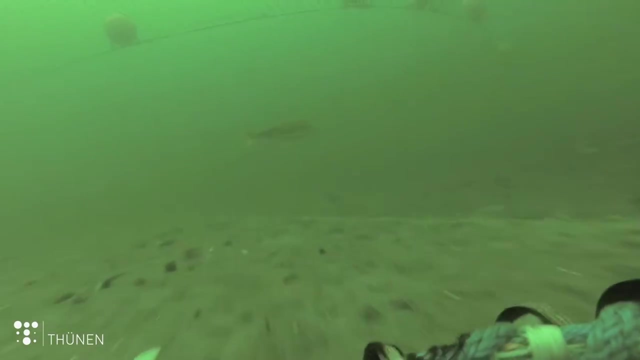 For decades, high-intensity, harmful trawling methods in various sectors of the fishing industry meant many stocks were overfished, damaging whole ecological communities In Europe. the reform of the common fisheries policy now creates a new trend, now creates a new chance for fish stocks and marine ecosystems to recover. 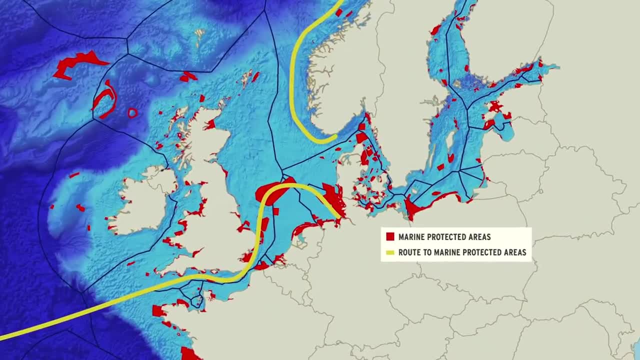 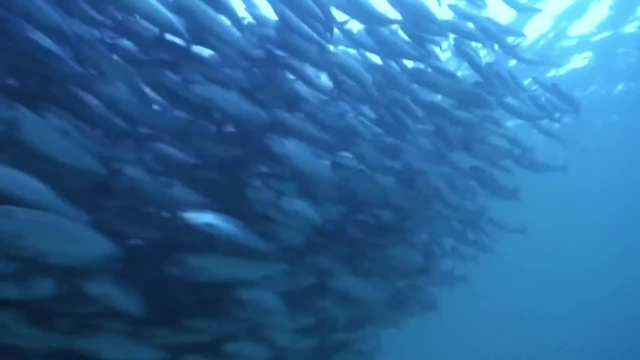 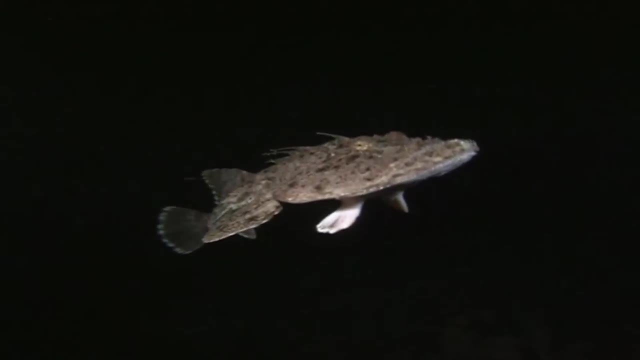 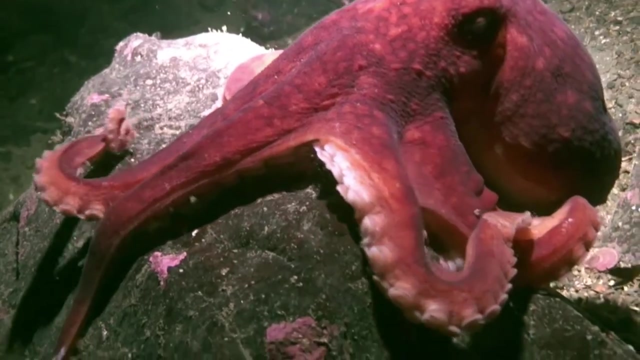 From the Atlantic, we travel along the deep trenches past the Norwegian coast, heading south. Shoaling fish like herring and safe are at home here. Another somewhat scary-looking inhabitant is the monkfish, a sought-after but endangered tablefish. Cephalopods like red octopus find places to hide between the rocks. 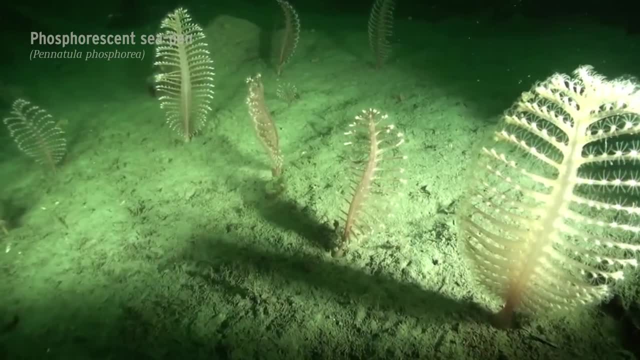 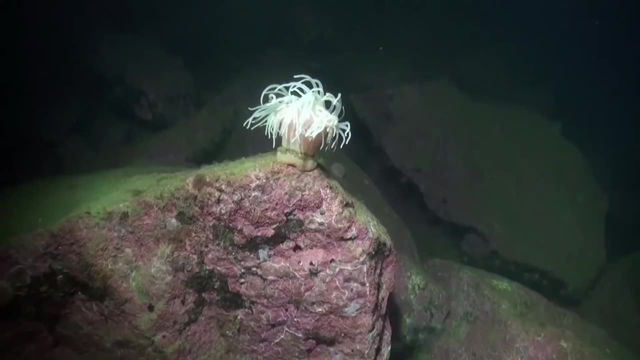 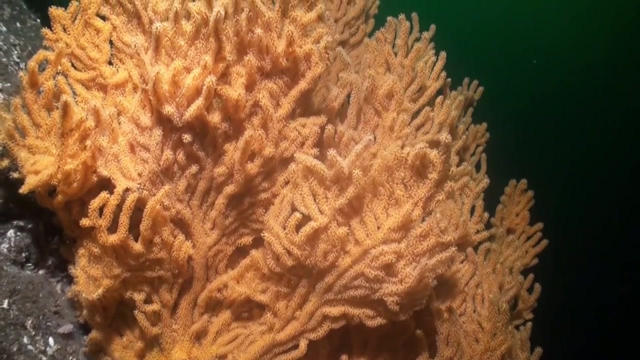 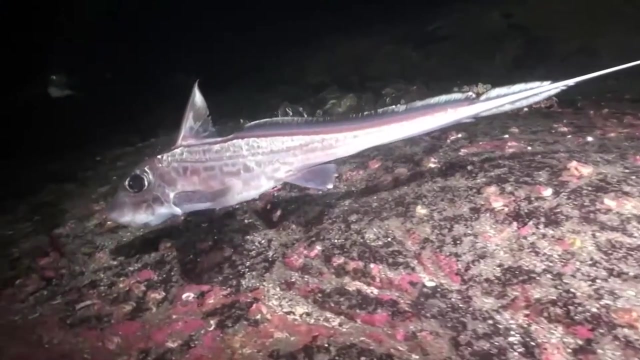 Sea pens are characteristic of a special, rare type of habitat: Sea anemones and rare cold-water corals like Paramericea, a deep-water fan coral, grow along the Norwegian continental shelf. Chimeras flit through the deep dark waters. 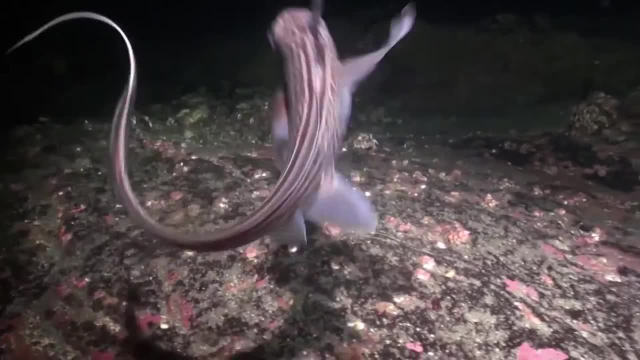 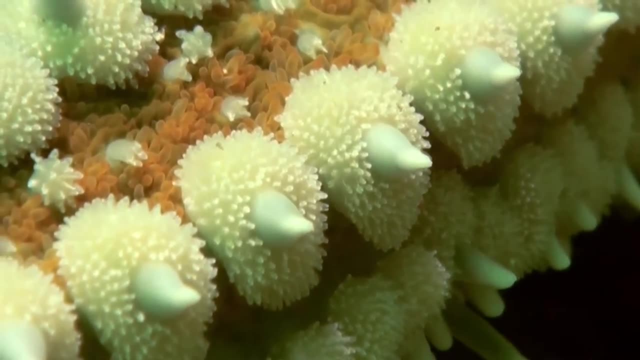 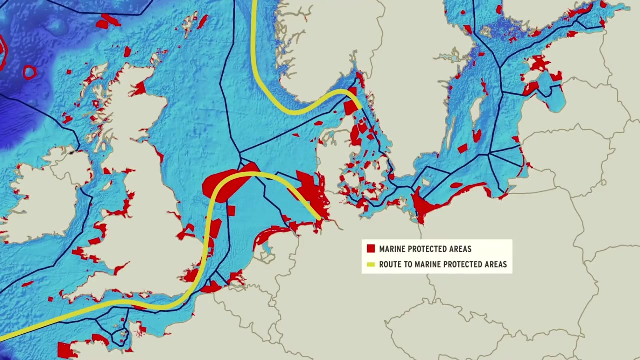 Marine-protected areas once again play an important part in conserving these fascinating species and the whole ecosystem. On we go through the Skagerrak and Kattegat to the Danish Straits, the only place where there is an exchange of water. 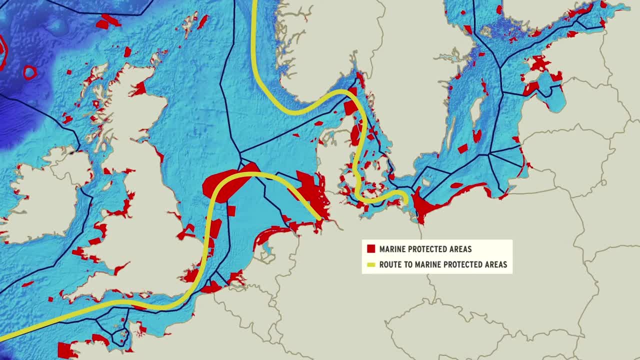 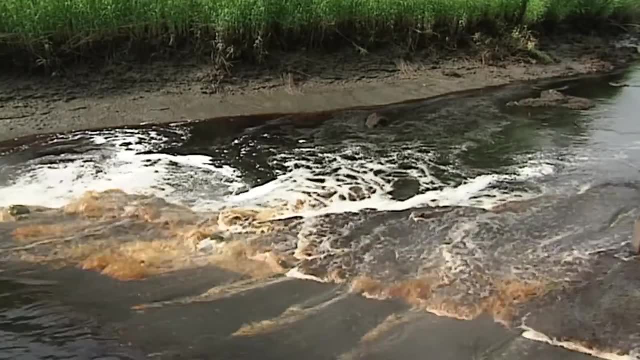 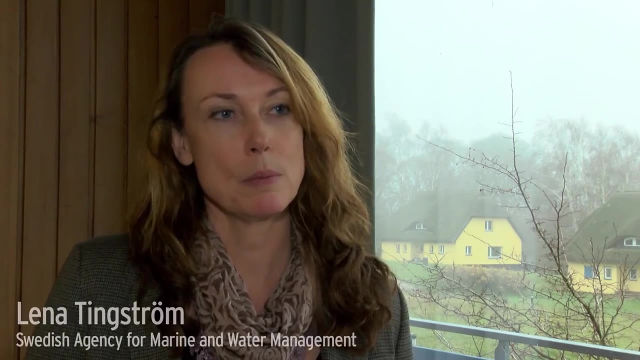 between the North Sea and the Baltic. All the surrounding states have created MPAs here. Despite these, nutrient and other forms of pollution from diffuse sources is still a widespread problem, And of course, the eutrophication situation in the Baltic Sea is a big problem. 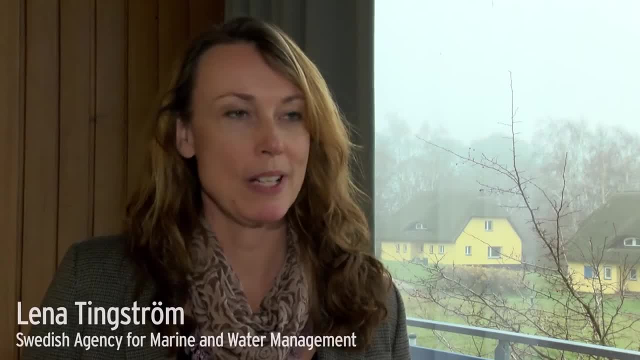 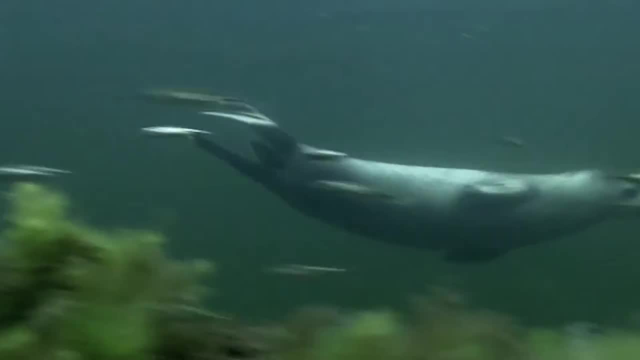 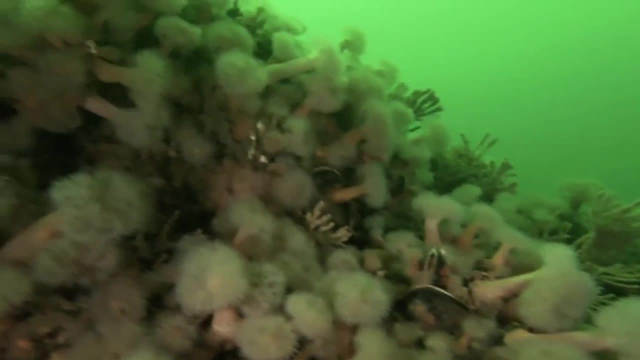 It's a big issue for us to address And that's not possible really within the separate marine-protected areas, so you have to work on a broad scale, like the Baltic Sea Action Plan. The Baltic Sea is a highly sensitive ecosystem, Improving its overall ecological status. 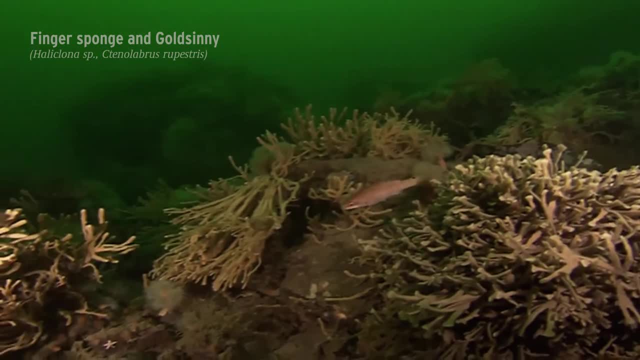 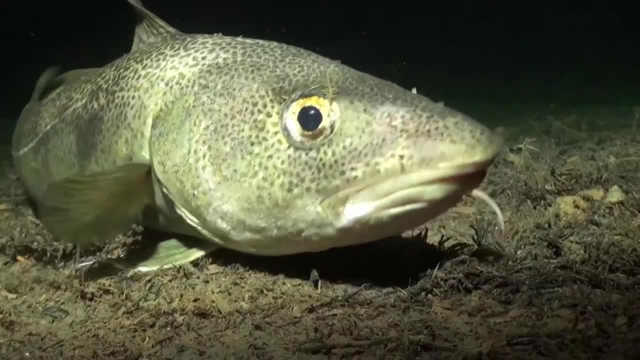 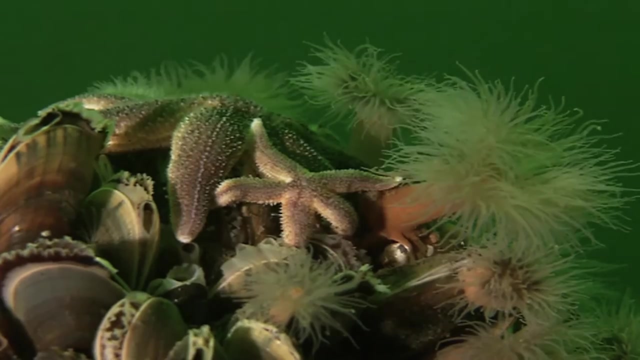 and sustainable management of the sea is the goal of the parties to the Helsinki Convention. under the Baltic Sea Action Plan, The network of Baltic marine-protected areas already takes in some 10% of the sea. This includes five large areas in the German Exclusive Economic Zone. 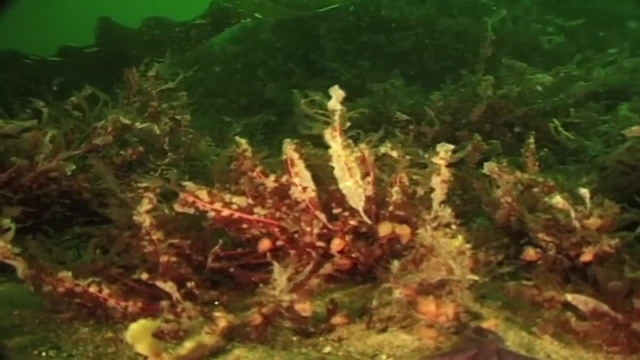 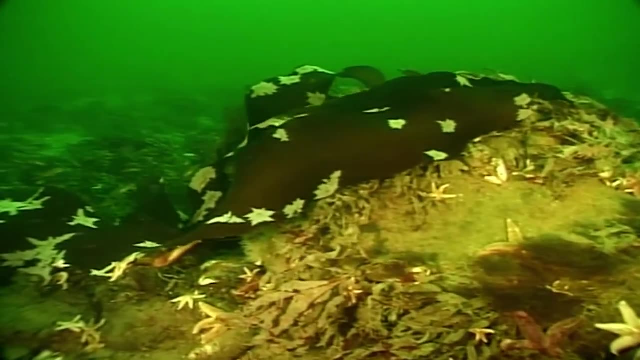 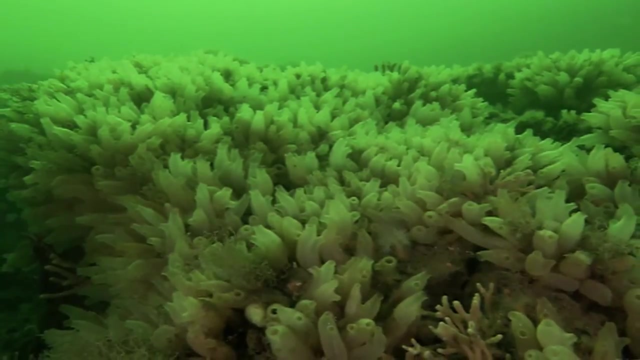 or EEZ. Blue mussels, red algae and kelps are characteristic of the Fiemann Belt and the Kadett Trench Sea. squirts are also found here Further east on the Odra bank. highly endangered eastern Baltic harbour porpoise. 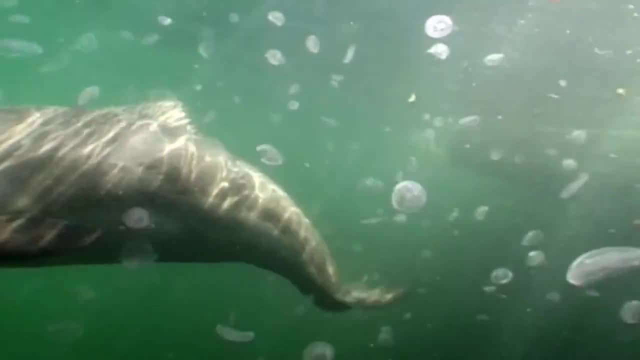 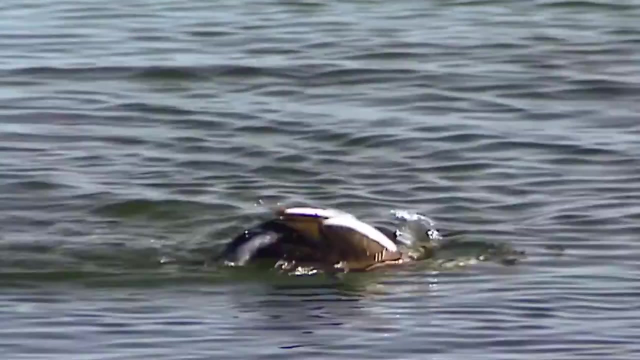 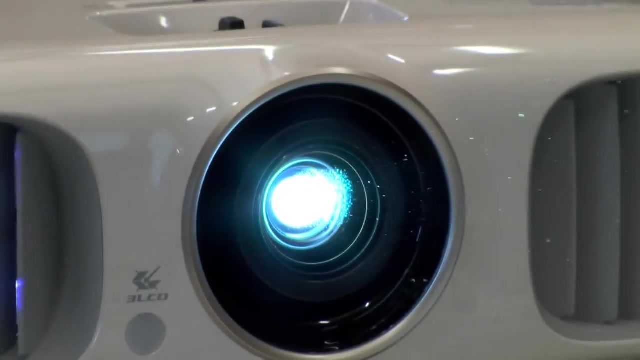 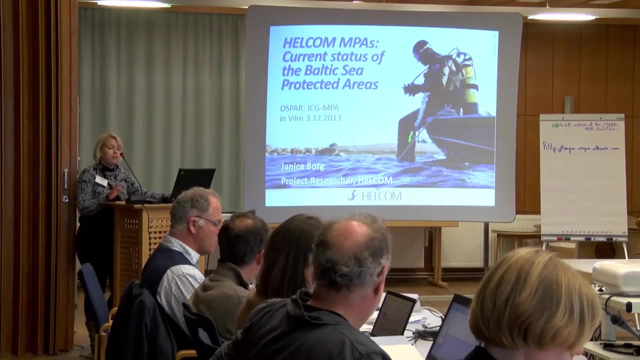 find a retreat. Long-tailed ducks and many other sea birds spend the winter here in internationally significant numbers. For the protected areas in the German EEZ, the BfN develops management plans and works continuously to improve the protection rules. The outcomes: 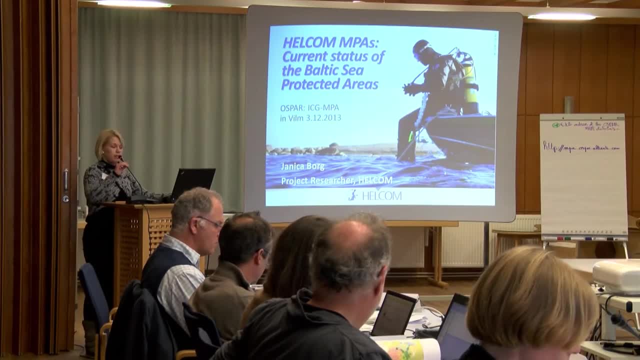 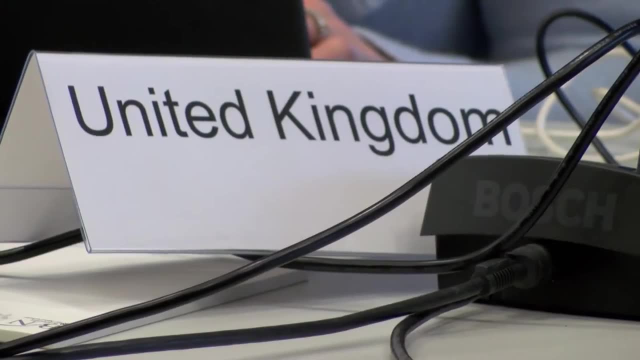 including rules on fishing in protected areas, are shared with other HELCOM and OSPAR party states to serve as examples in their own work, For example in the OSPAR Working Group on Marine Protected Areas, which is chaired by Germany through the BfN. 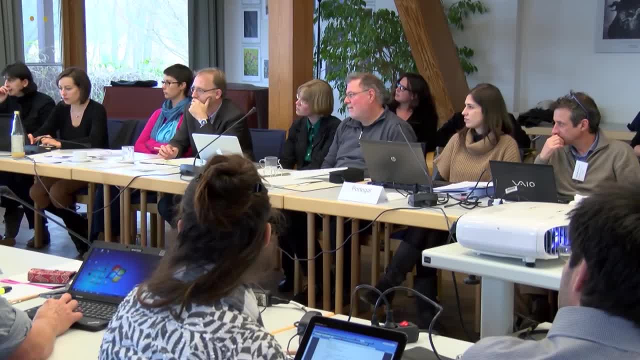 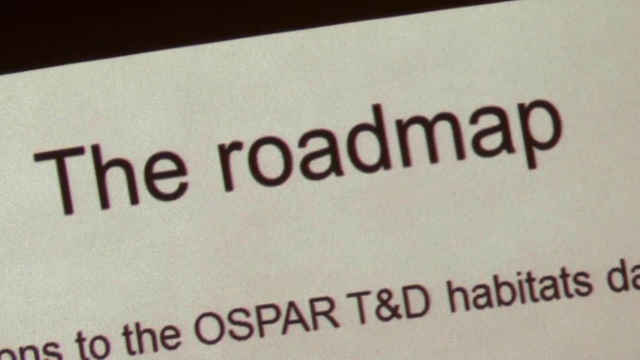 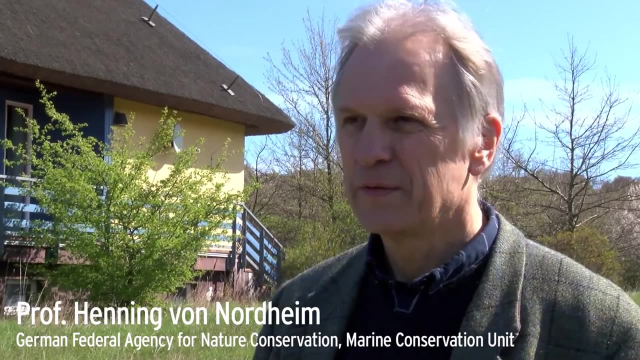 But there is still much to be done before valuable marine areas can enjoy protection worldwide. The first key step will be to finalize the EPSOS process that CBD has started. That means other parts of the world which have not yet identified their ecologically important areas. 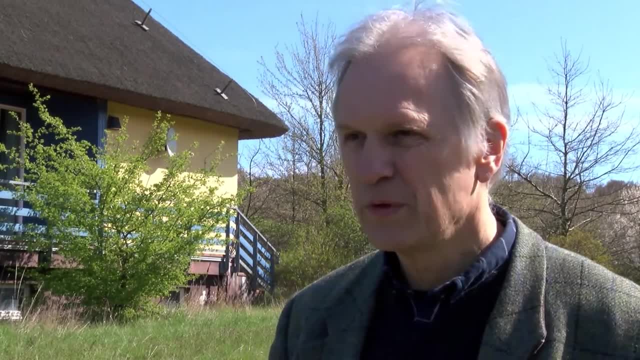 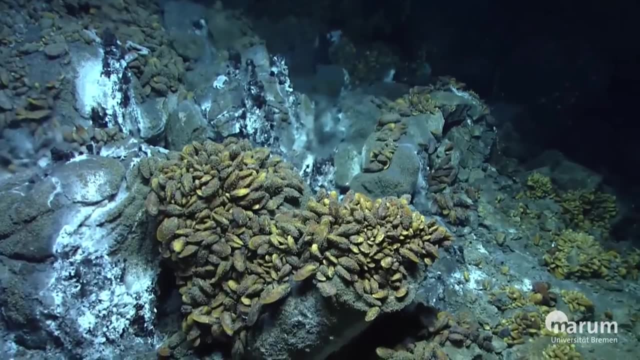 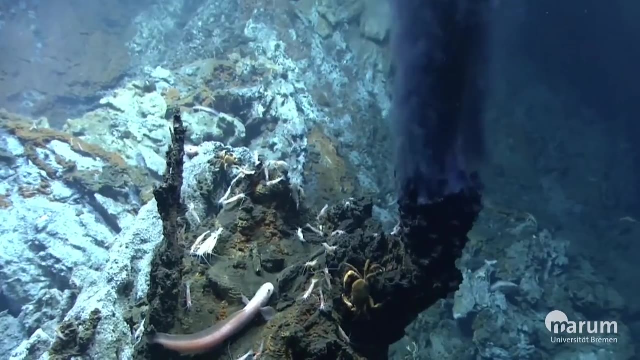 should do so as quick as possible. I'm talking about the Antarctica, for example, but also in the Arctic and other parts. there are some pieces missing in this overall assessment. The second, and even more key step would then be to identify within those ecologically important areas. 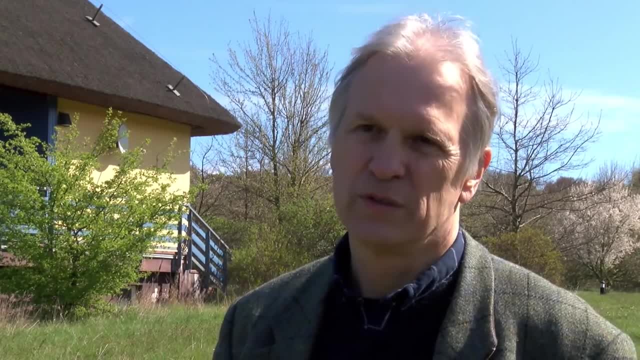 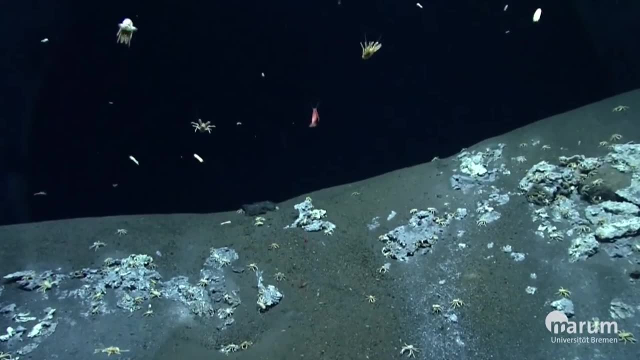 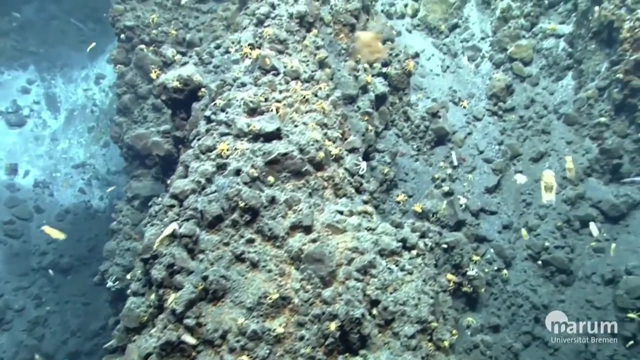 those sites that should be granted an international conservation status, a protection status. And to grant such a status, we need a third step to be fulfilled, and that is a global agreement on UN or on the level of UNCLOS, that allows us to protect and conserve.